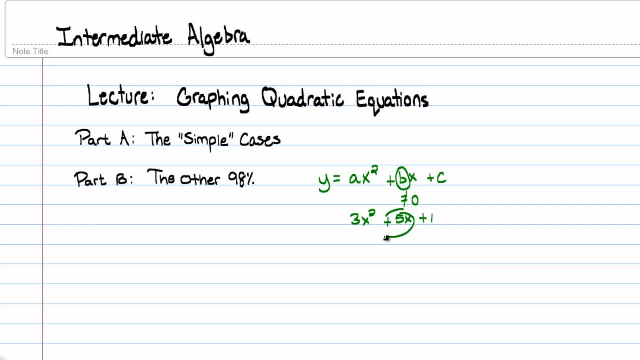 But all the other cases where we don't have a term with an x in it are treated in part A of this lecture. Now to begin this lecture, which is for quadratics- probably the most important lecture you'll see for graphing quadratics. 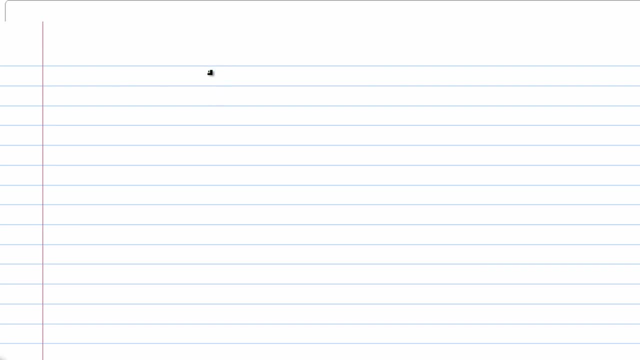 I want to introduce something that will seem very foreign to most people. Most people have never seen this style of graphing a quadratic equation, but I like to teach things that are more about common sense than about memorizing. So one thing I want you to note. 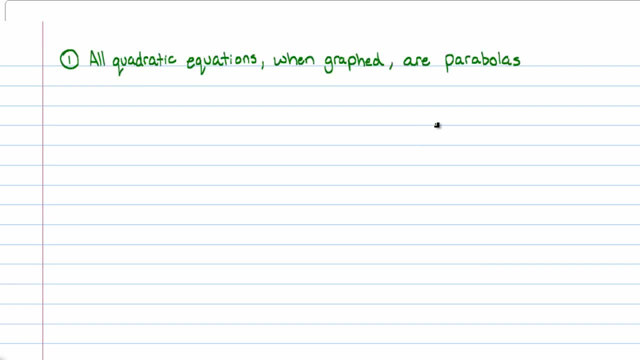 Actually a few things I want you to note. First thing: all quadratic equations, when we graph them, they graph as parabolas. And those are these objects right here, right, These kind of. some people call them V-shaped, some people call them U-shaped. 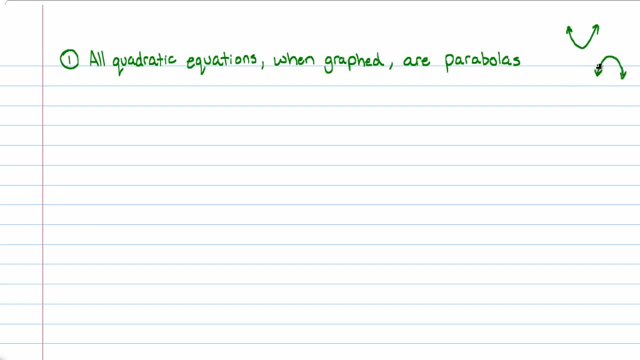 I'd probably call them a U-shape as well. They're an ever-widening U-shape. They either open up or they open down, and later on in mathematics you deal with some that open left and right. But for now let's just think about this. 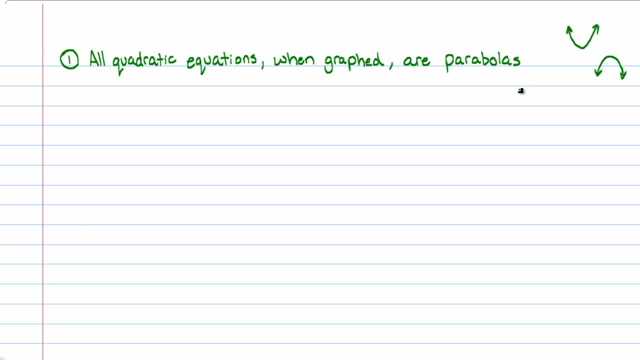 That they're all kind of these widening, widening U-shapes. The second fact that I want to mention that should be common sense is that all parabolas must eventually hit the y-axis. And that might not be super common sense yet, but let's just take a look at a graph here. 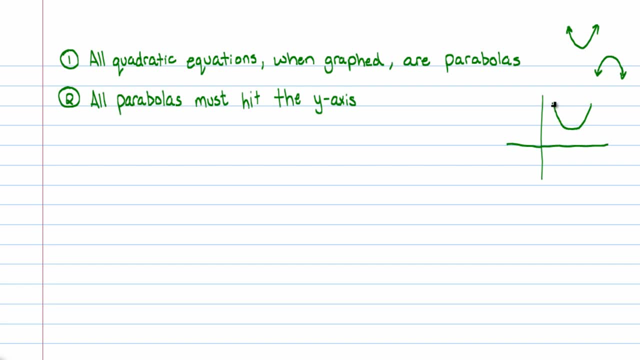 And I'm going to graph a parabola right here Now. remember, parabolas go ever, ever wider. In other words, this keeps going out to the left, But eventually it's got to cross this y-axis. It's just going to happen. 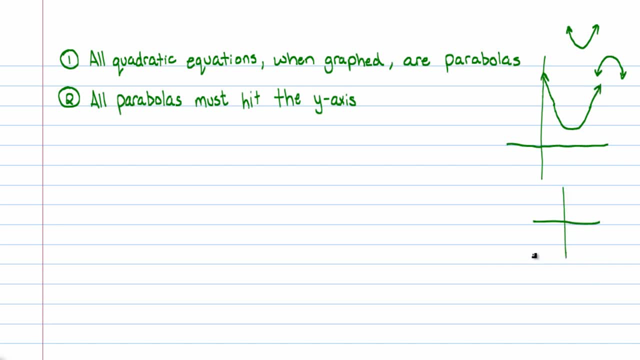 Same thing. if you graphed a parabola upside down, Let's say we graphed it way over here And it's very skinny. Even if it's very skinny, eventually it'll hit the y-axis Eventually. So at some point, a parabola- it doesn't matter what the parabola is. 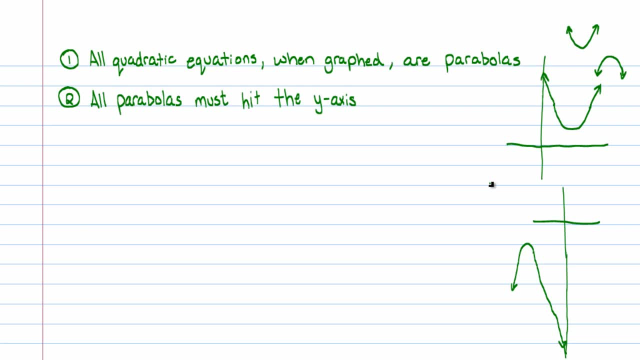 eventually, all parabolas must hit the y-axis, So that's something that I want you to kind of think about. Spend some time thinking about objects that just go ever wider like that, And you can probably convince yourself that they will all encounter. 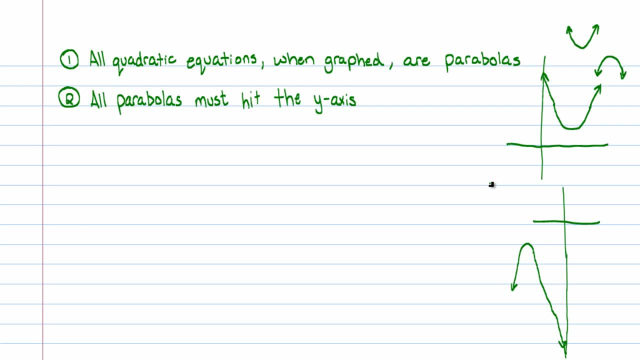 or run into or intersect the y-axis. The next thing I want you to kind of think about is that all parabolas, since they have a U-shape to them, if that U-shape- And I'll graph this out kind of like this: 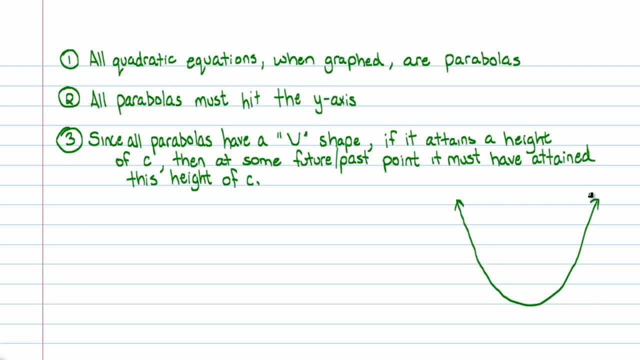 You can think about Pause it after I talk about it, whatever, But if this U-shape attains a height of, let's say, let's just pretend this is a height of 5.. Okay, So I don't know what the x-value is, but I know this height is 5.. 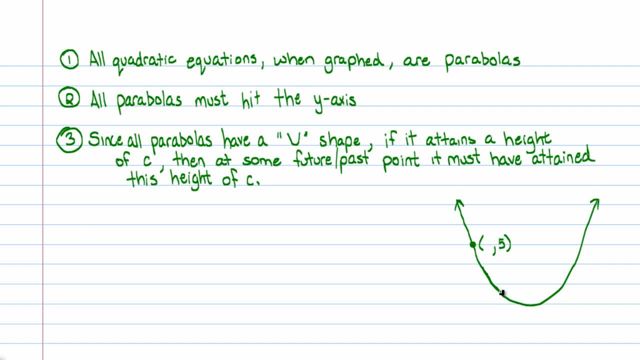 That because it's a U-shape at some point in the future or in the past. if we're going backwards, it'll reach up to that height of 5 again. I just don't know the x-value for that. I don't know the x-value for that. 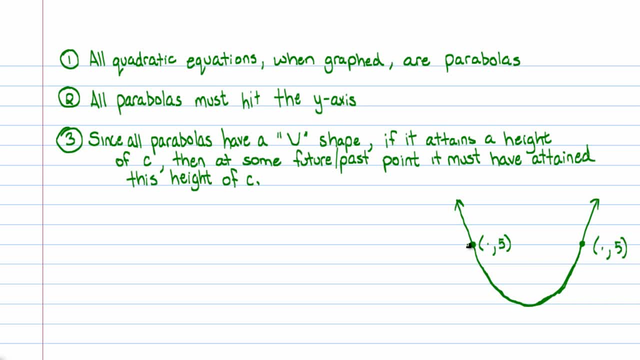 But the fact is it's a U-shape Symmetric. If it reaches a height of 5, it should reach a height of 5 again. There's only one exception to this: If you're at the very bottom, you're not going to reach that very bottom again. 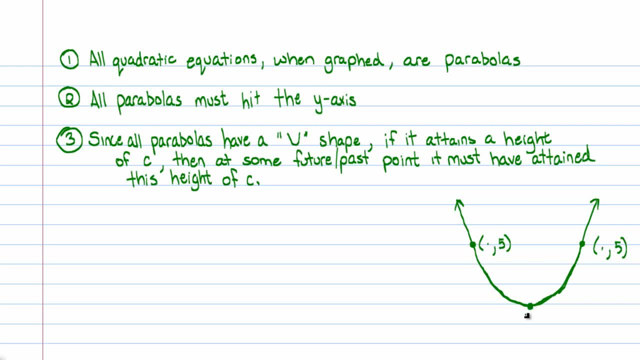 In other words, there's no other point that reaches this bottom except for the bottom itself. But if you want to reach this height right here, well, there's a symmetric point over here, And in fact that's what we call these. 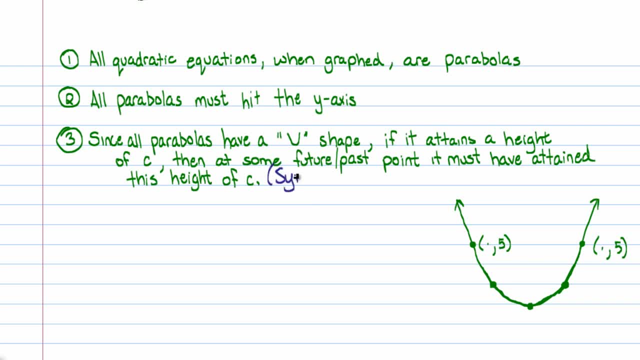 We call these symmetric points. So every point, except for the vertex, every point on Every point on a parabola, has a symmetric point, Point of symmetry. And, by the way, that symmetric point can be found just by looking at this axis of symmetry. 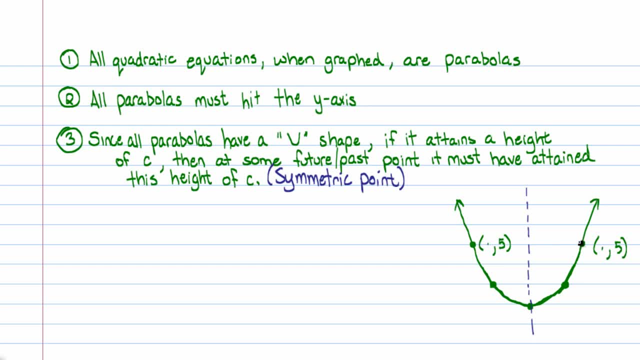 It's a mirror image, right? So you have to have, You have to be at that height again. I want you to really think about that If you say, oh, I totally get it right now, I promise you when we start doing examples. 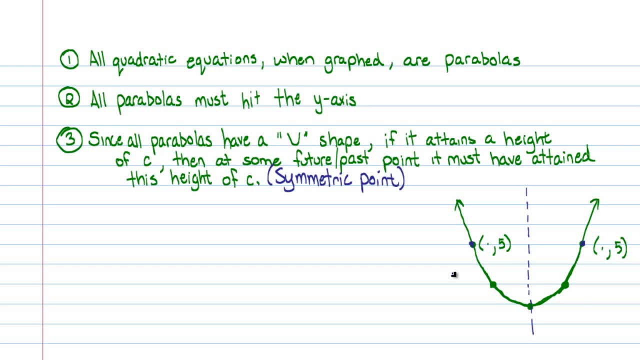 that you might go. what the heck is he talking about? So I really need you to think about this. That listen, you've got a U-shape. You are at about five feet tall That then later on it will have to reach five feet tall again. 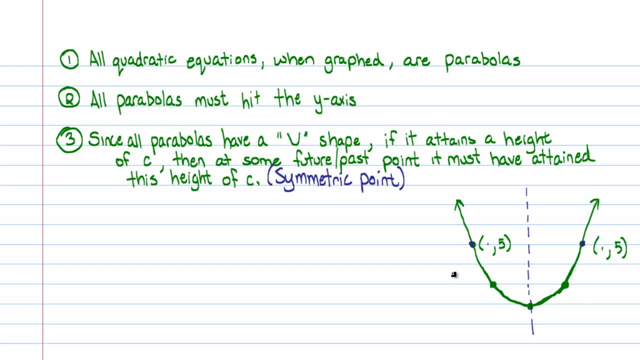 because it's just going to curve down and come right back up. Probably the most important part of this- and actually the reason why I'm teaching this method- is that when you want to graph a parabola, you're really looking to graph the vertex. 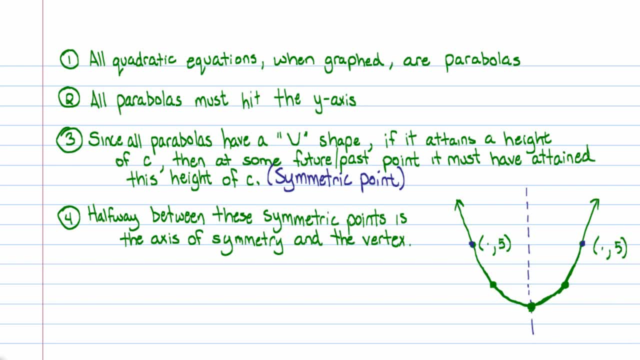 the lowest point or the highest point. In this case, with this parabola that I've drawn, since it opens up the lowest point. However, if it opened down, I would be talking about finding the highest point. But anyway, finding that vertex is the most important thing when you're trying to graph. 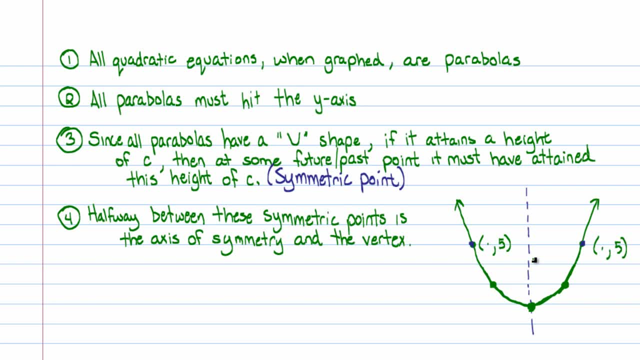 a parabola And in fact, for applications, it's always what we're looking for, almost always what we're looking for. So halfway between these symmetric points is going to be the axis of symmetry, where that vertex lies on. So if you take a look at this symmetric point at a height of 5 that we 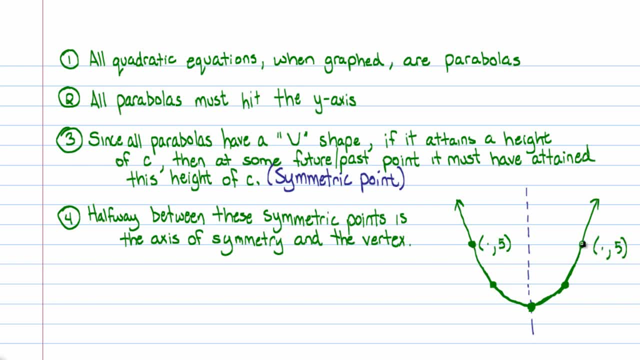 said earlier, and its other symmetric point, which is also obviously at a height of 5, halfway between these, must be the vertex. It's a U shape, Halfway between any two symmetric points has got to be the vertex. So, if I know, let's pretend, for example, that this x-value is 0. 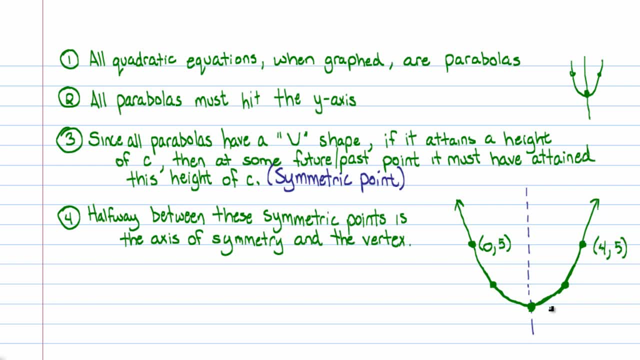 and this x-value here is 4, then I happen to know the x-value for the vertex must be 2.. It's halfway in between those two x-values. Alright. the only problem is we don't know the corresponding y-value, And that sometimes is. 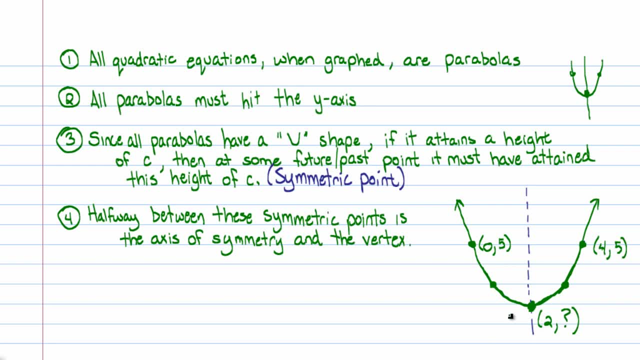 important in applications. It's very important in graphing. So the last step, really the fifth idea here, is that we're just going to plug this x-value into the original equation to find out the y-value. Now you should be writing this down. 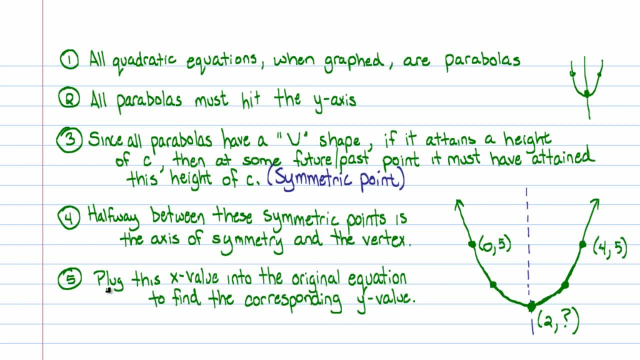 If you're in a class- my class, I don't care. It doesn't matter if you're in my class or somebody else's class. You should be writing this down. Just watching a video online is not going to educate you. What's going to educate you is you participating in this and actually 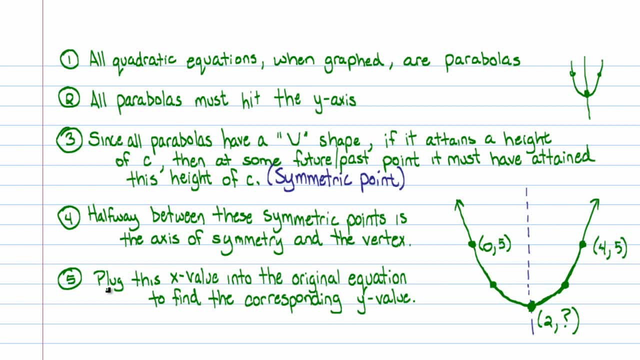 thinking and trying to be a scholar really and educate yourself. So please write this down, Have it available, because I'm going to just not refer back to these things, I'm not going to hop back to this, I'm just going to start doing examples and graphing a bunch of things. 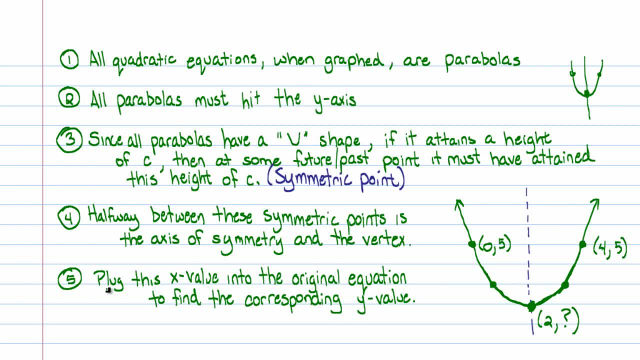 One thing I do want to mention, though, is that this method really is great if you have something of the form y equals, or I shouldn't say something a quadratic equation of the form y equals ax squared plus bx, And then you might have a c on there or not, It doesn't really matter. If you do have a. 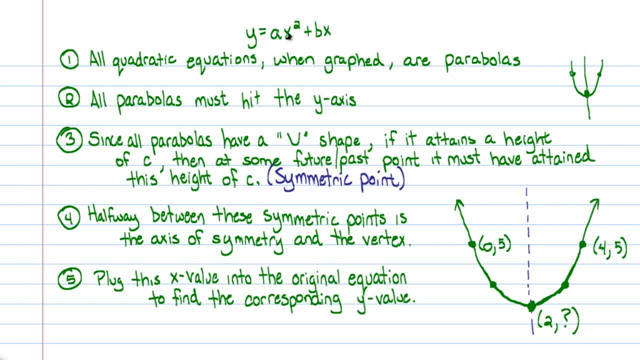 plus c. that's good too. You could use it for that as well, But it's not good really if so I'm going to put this in red. so don't use if you have something like y equals just an ax squared or y equals. 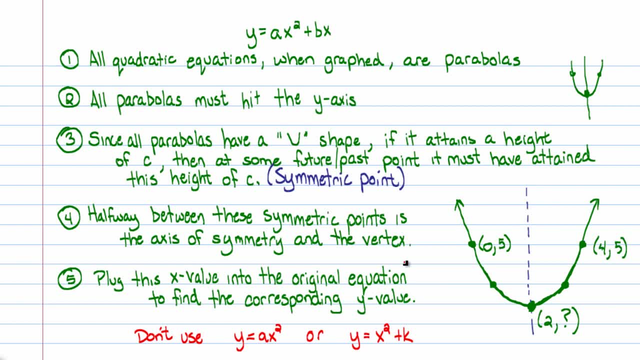 like an x squared plus k. Those are way too simple to use this, this method on. These are the simplest kinds of quadratics you can graph. If a is three, it looks like the regular parabola, but it's three times. 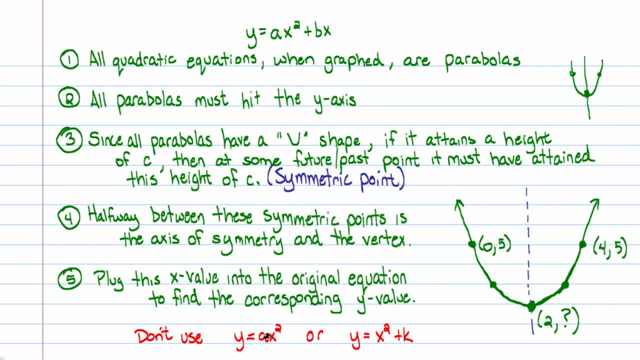 it's stretched by a factor of three. If a is one third, it looks like the regular parabola, but it's compressed by a factor of one third. In this other case, right here, if k is five, it means it looks like the regular. 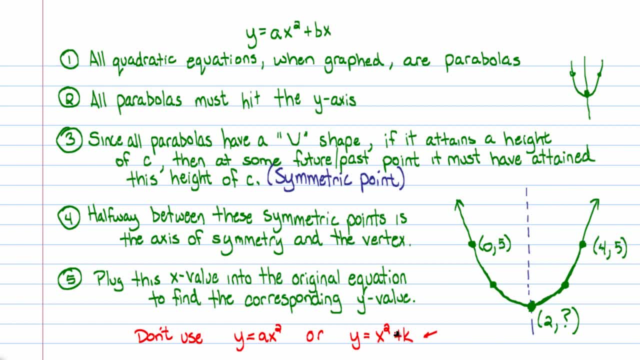 parabola. it's just been lifted up five units. Those are very fast to graph, but these ones up here, let me go ahead and point at it with a green pen, these ones right here not so much, Those are actually been shifted and it's very. 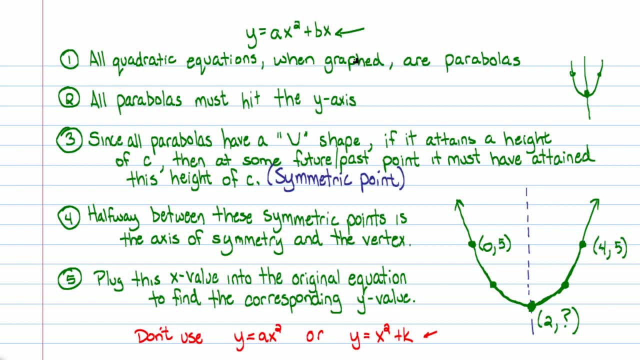 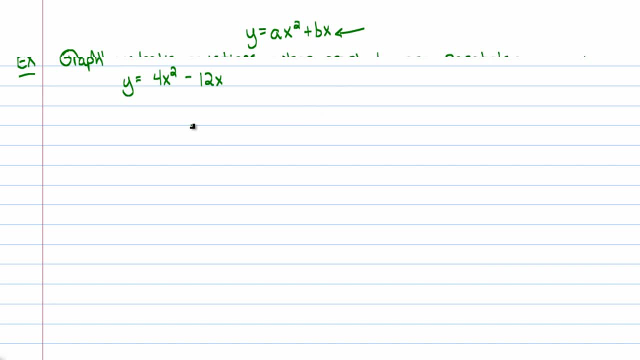 difficult to figure out which way they've been shifted. In fact, let's go ahead and do an example here. Let's graph: y equals x squared minus 12x. The first thing I'm going to mention is that this has got got to have a y-intercept. 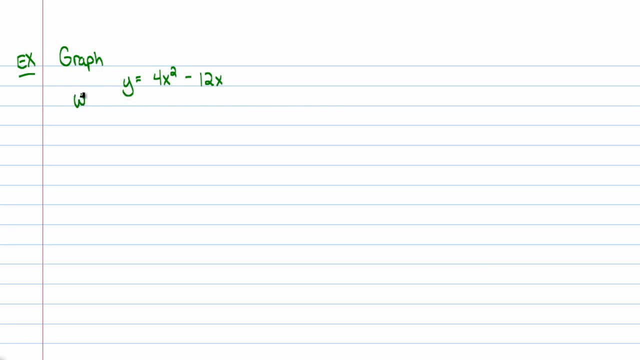 It's a parabola, right? So what is the y-intercept? When are we going to hit the y-axis? That should be a question mark there. So the y-intercept. the reason why I like this method so much is that the y-intercept is the fastest intercept to get, because 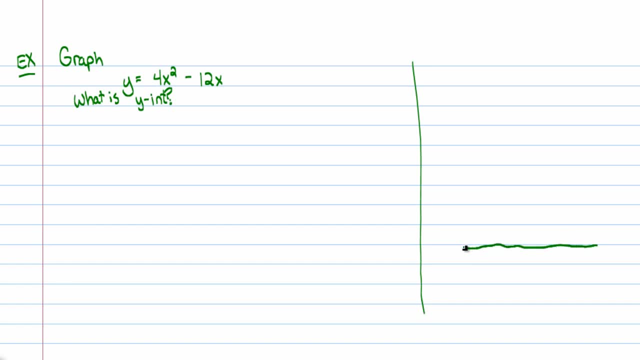 all you need to do is to notice that on the y-axis itself, which is what we're asking, where we hit the y-axis, on the y-axis, all the x values are zero. So just let x equals zero. If you let x equals zero up here, you find out that y is also zero. So I guess the y-intercept. 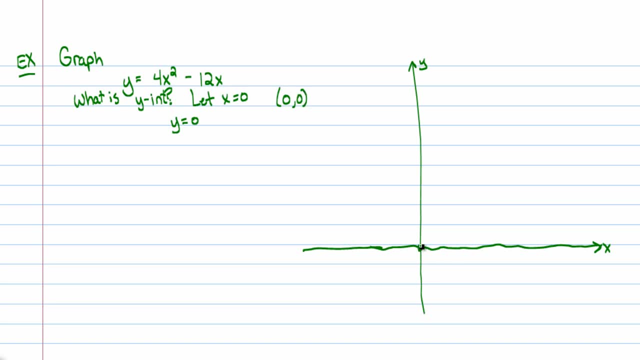 just occurs at zero comma zero, And let me draw that in a different color, an annoying color. there we are. Now that we have that and we've found that out, let's go ahead and ask ourselves: well, I know, it's a u-shape. 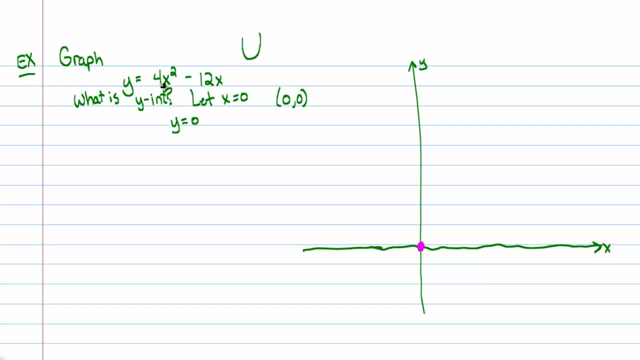 it's like it might open up. well, actually it does open up because it's a positive number there, but we I don't really usually talk about that. It either opens up or opens down. The fact is it's it's a u-shape. So if I hit the height of zero, 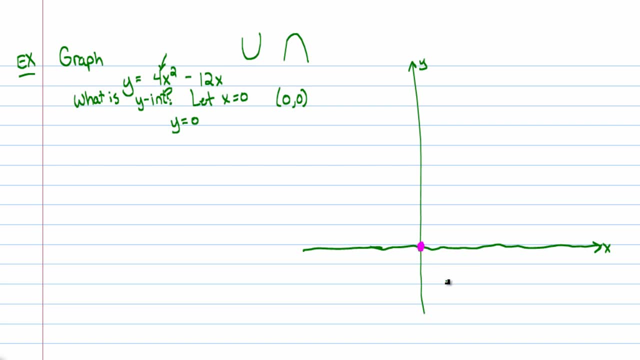 at some at this point, then later on I should crawl right back up to the height of zero again, Or I might crawl right back up the height of zero to the left, but it doesn't matter. The question is, when is the height? that's how I'm. 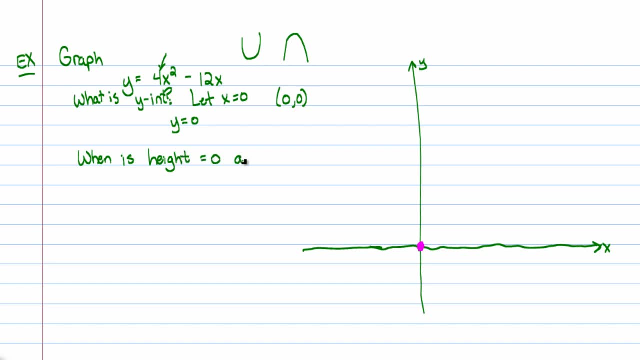 gonna call it here equal to zero again, Because I want you to think about this in common sense. Like, listen, it's a u-shape. when are we gonna be at that height again? Well, you just go ahead and let y equals zero. Alright, so here we go. 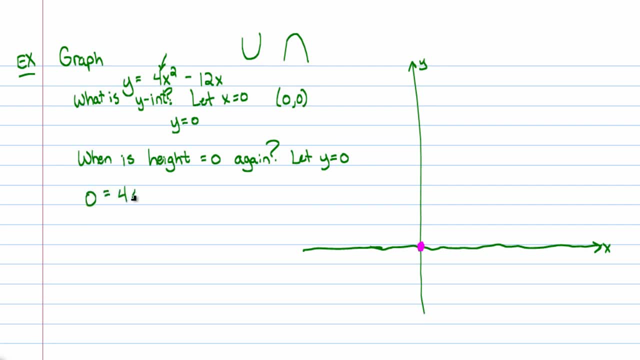 I'll let y equals zero in my original equation and, lo and behold, I get this beautiful result. I have a quadratic equation that I can solve because I know to how to factor quadratics. I know how to solve quadratics by extraction of. 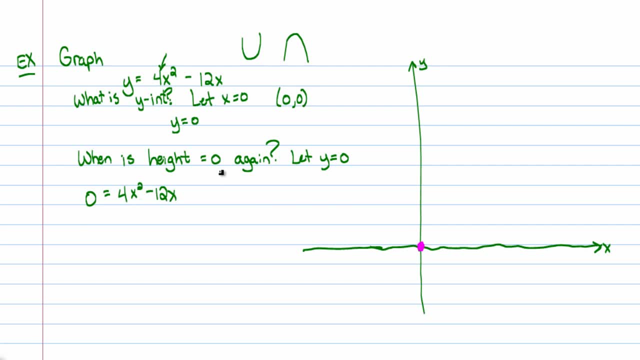 roots. In this case it would be factoring. In fact, all these cases it would be factoring. So let's go ahead and see what we can factor out of the right hand side. Both those terms have a 4 and an x in common. That leaves me with x. 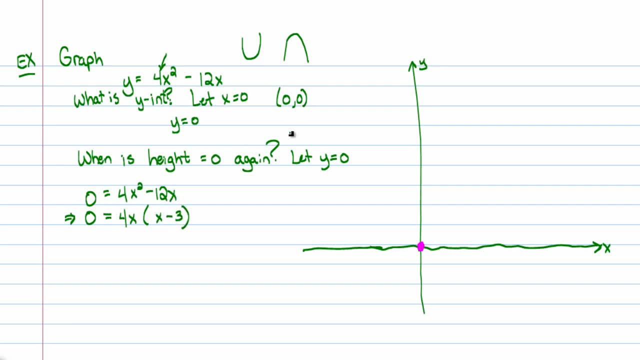 minus 3.. So it tells me I'm at a height of zero again, when that first object is zero, or when the second object is zero, or in other words when x is equal to 3.. Okay, I could play that. 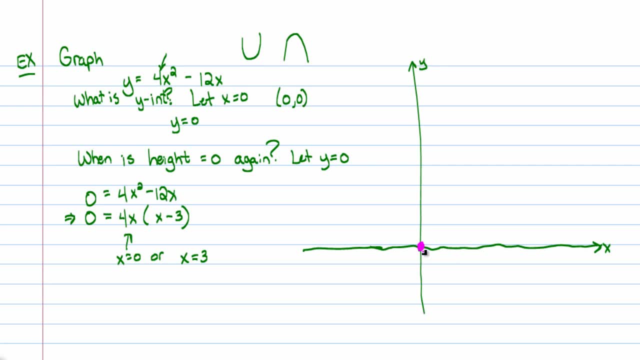 game. So I'm at a height of zero when x is equal to zero. but I already had that written in there. and I'm at a height of zero when x is equal to 3.. I'm at a height of zero when x is equal to 3.. 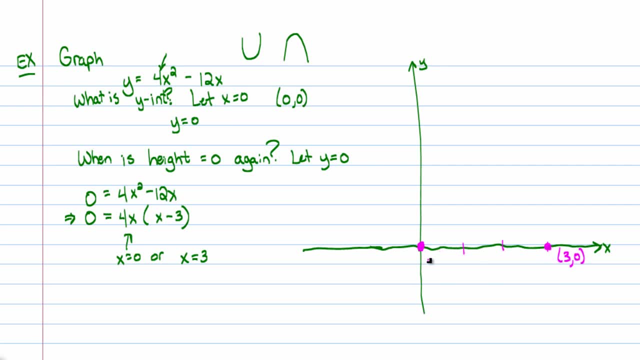 Those are my symmetric points. Those two points actually exist on my parabola. Halfway in between must be the axis of symmetry. right, It's a, it's a u-shape, so it's like we found these two points So halfway in. 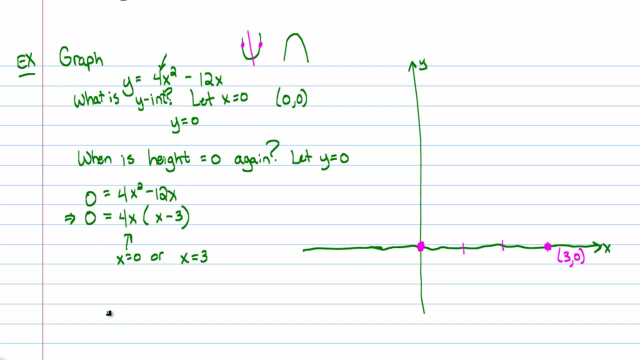 between has to be the axis of symmetry. So let me just write axis of symmetry and remember it's a. the axis of symmetry is a vertical line. So remember equations for vertical lines are of the form x equals and it's halfway in between 0 and 3, so it's the average of those two numbers, 0. 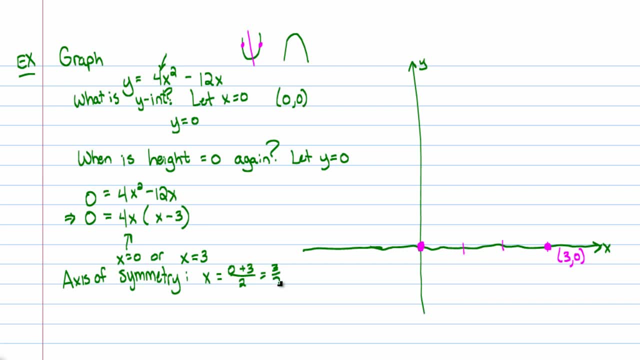 plus 3 divided by 2, or in other words 3 halves. I'm going to create a little dashed line here at 3 halves, which is 1.5.. x equals 3 halves, and I know that's where. 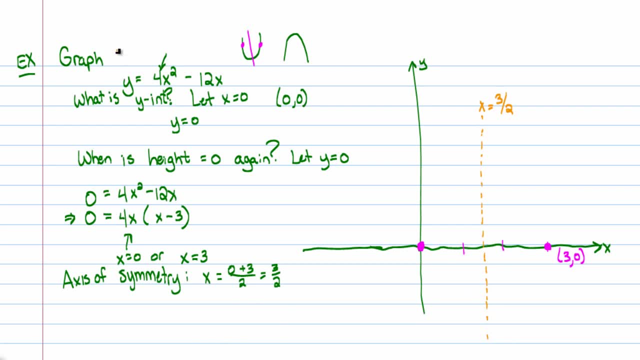 the vertex is going to be. The vertex is going to be at 3 halves comma something. That something is a y value. I just need to plug in 3 halves into my original equation to find it. Well, let's see, y is equal to when I substitute in 3 halves here for x. 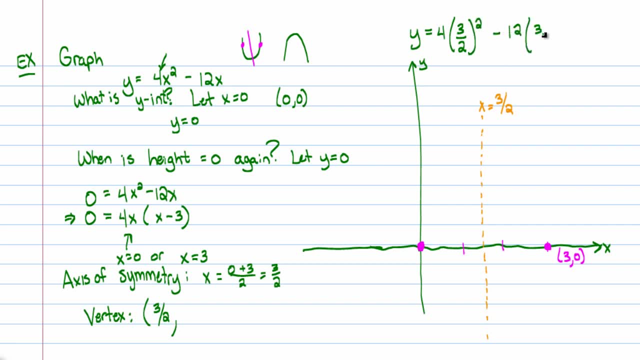 I get the following: well, let's see, 2 goes in, that 12 six times. so that's nice. and when I square this well, I better just square it because I don't want to mess people up here. so this gives me 4 times 9. fourths minus 6 times 3 is 18, and the 4 and the 4 will cancel. 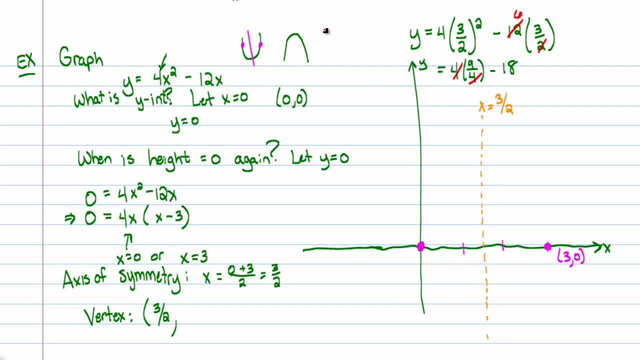 right, 4 over 4 is just 1, so that'll be 9 minus 18,, which is a negative 9.. Now I didn't really leave a lot of room for a negative 9, so I'll just pretend as though that. 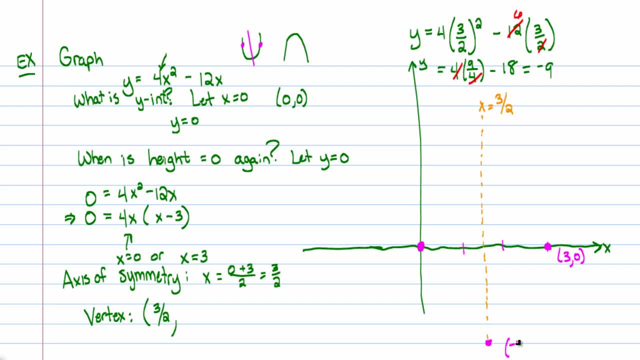 point right there is at a height of negative 9,. remember, the x value is at 3 halves and the y value is at a negative 9, and now I have three points. very easy to graph a parabola once you have three points. 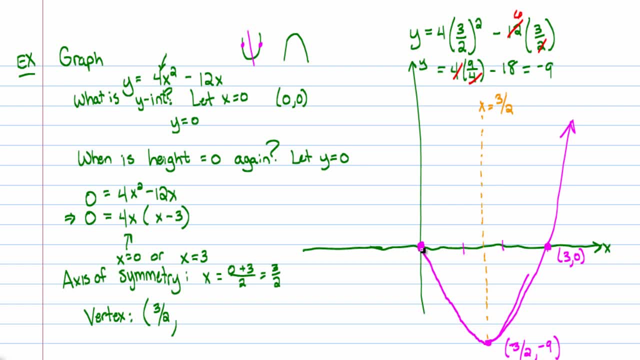 If you can draw straight on a digital board here, something like that. So to recap what just happened, because you might just go what the heck just happened To recap, I just asked: when am I hitting the y-axis? Well, let x equal 0,. okay, we did that, we found out. we hit the. 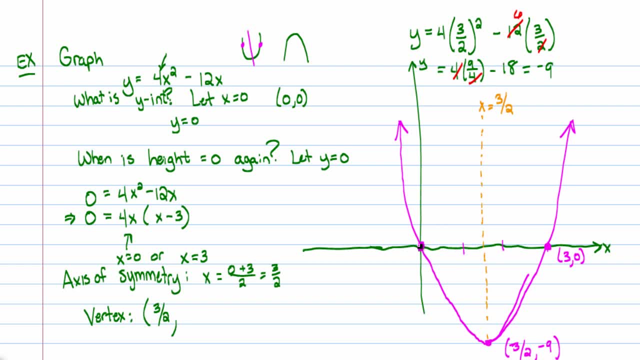 y-axis at 0,. okay, great. so I hit the y-axis at a height of 0, when am I at that height of 0 again? In other words, when can I be at that symmetric point again? So we let y equal 0 to find out, basically, when we're at that height of 0 again. 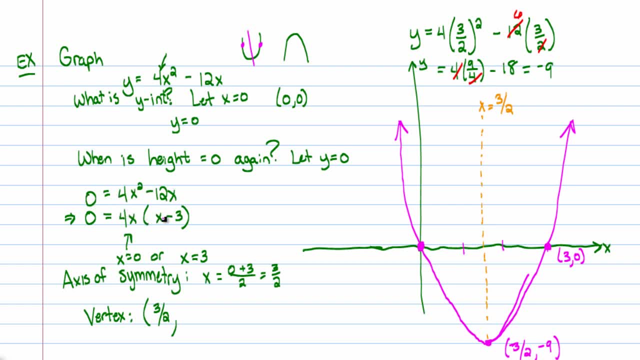 and we solve the corresponding quadratic equation, You find out that it happens that the height is 0 for this parabola when x is 0 or x is 3, so that's what I plotted here. this is: x equals 3,, the height is 0.. Halfway in between is the vertex. 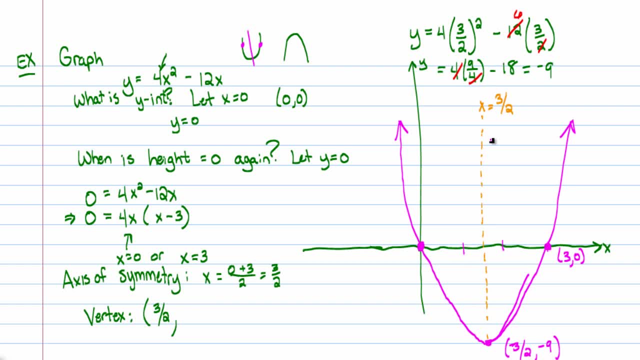 so I just found the halfway point between 0 and 3, that's pretty easy, that's arithmetic right, And then I plug that value in to the original equation to find out what the corresponding y value is for the vertex. 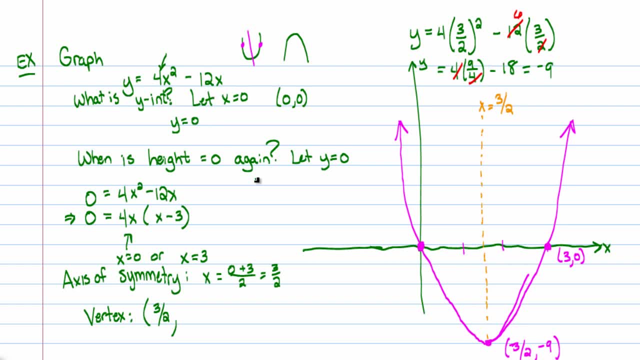 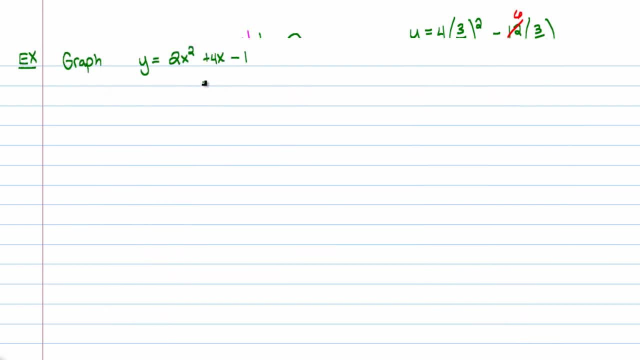 Now this may seem like a lot at first, but trust me, you get good at this. You can graph a quadratic equation in no time flat. Let's do a few more. This is an interesting one. Graph y equals 2x squared plus 4x minus 1.. I always start just by asking myself: 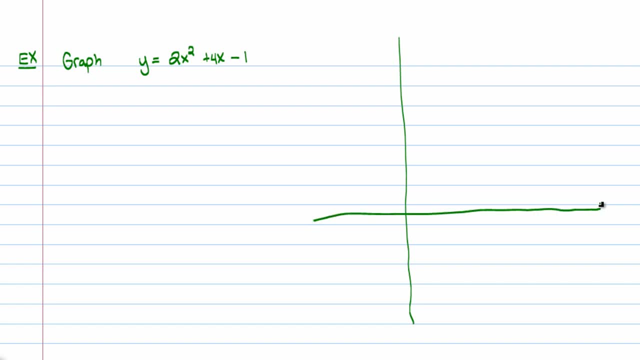 because I know it's a parabola because of the x squared. so I ask myself: when am I hitting the y axis? So where? well, maybe I should say: when do we hit y axis? Because it's got to happen? It's not necessarily true that we hit the x axis because we could have a parabola that looks like: 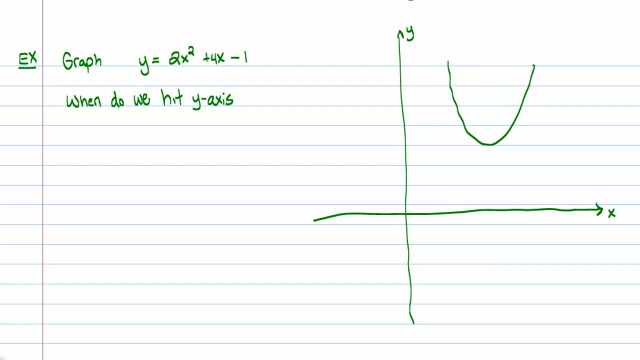 this, It would never hit the x axis, but eventually it widens out enough to hit the y. So I don't really start by asking when am I going to hit the x axis? I always ask when am I going to hit the y axis? Well, that means let x equal 0. So I do that here. I'll let x equal 0 and I find out. 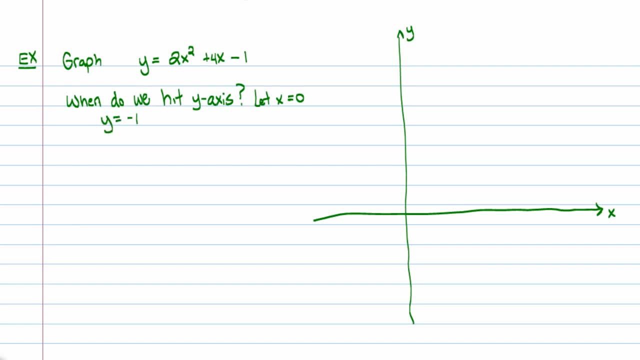 that occurs at negative 1.. You know how easy that was: Cover up these things with x's, the terms that have x's in them, because they're just 0.. I get y equals a negative 1.. I'll plot that point. 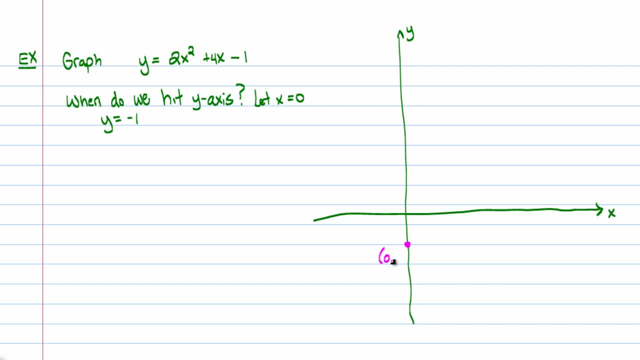 Let's pretend this is the height of negative 1, so it's 0 comma negative 1.. And now I'm just going to ask myself: well, I want to know where's the symmetric point. Is it to the right, Is it to the left? So when are we at a height of negative 1 again? 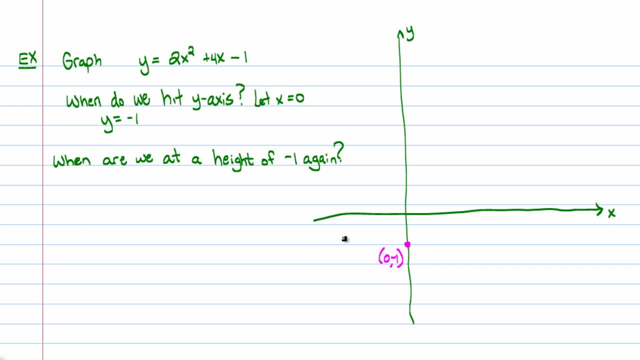 It's such an important question. When am I going to be at that height again? It's like a roller coaster. Am I going to roll down And come right back up and it will occur here, Or am I going to roll down this way and come back? 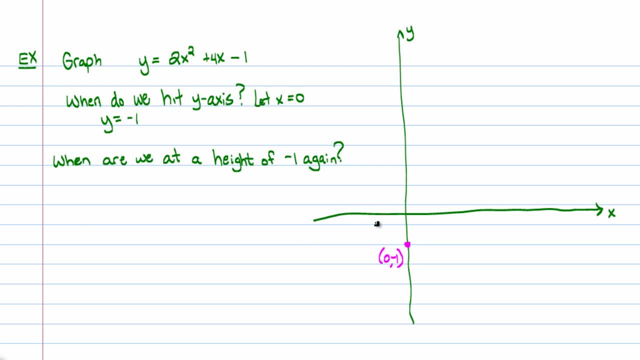 up and it will occur over here. That's an important question. So you let y equal negative 1, because you're asking: when am I going to be at height of negative 1.? So go back to the original equation: Let y equal negative 1.. Now a lot of people get intimidated by this step because 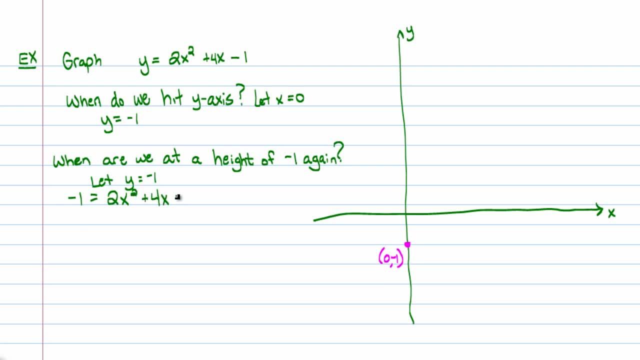 they think: oh man, I have to solve a quadratic equation. But guess what happens? And this always happens. There's a lot of fluke here. This always happens. I'm going to add, because I see I have two versions of x, two different powered versions of x, which means I have to move everything to one side of. 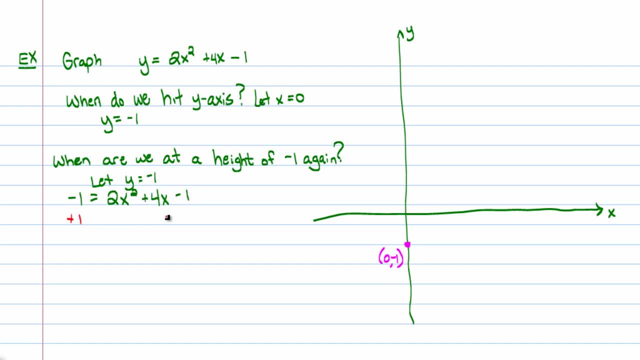 this equation. So I'm going to add 1 to both sides, And when I do that, I get this beautiful. 0 is equal to 2x squared plus 4x. Notice: there's no constant left over there. There's no constant. 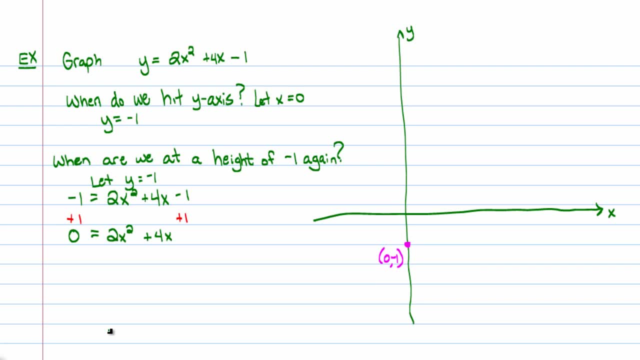 term. That will always happen when you use this method. Both those terms have something in common: The 2 and an x. So I'm left with x plus 2.. And this 2x times x plus 2 is equal to 0 when x is 0 or x is a negative 2.. 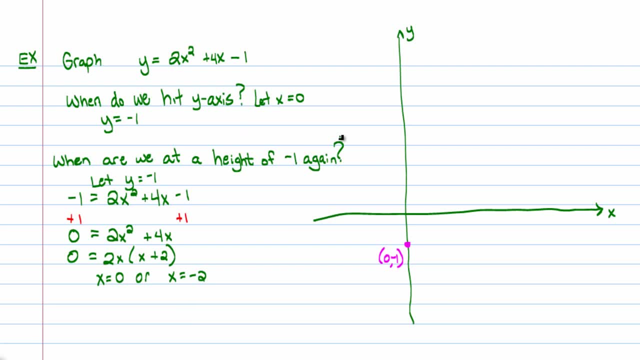 So in other words, I'm at a height of negative 1 again, when x is equal to 0.. Well, I already have that plotted. There's x equals 0, height is negative 1.. So I have one. So I hope this isn't going to prove Virtex. 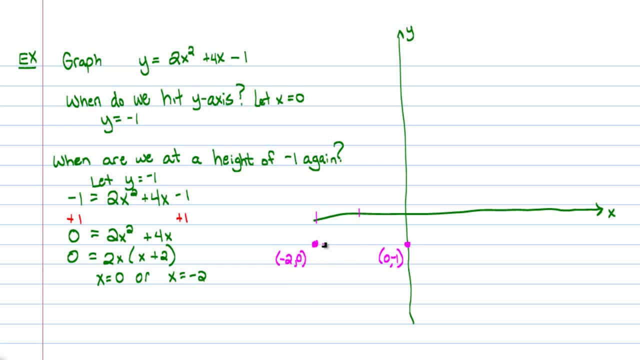 I go from 0 to 0 and x to 0.. I'm about to get an x that is negative 2.. Or x is negative 2.. So I have my symmetric points Halfway in between. these points is going to be the vertex. 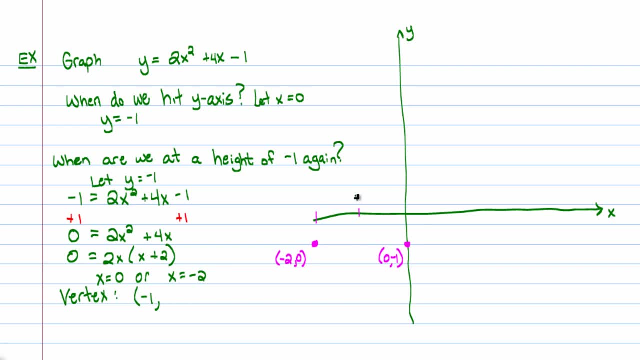 So let me just label that on here. I'll just type or I'll write in vertex this: you should really draw in an axis of symmetry that occurs at that halfway point. you should label it too. this is x equals negative one. that's the vertical line there. and now all we 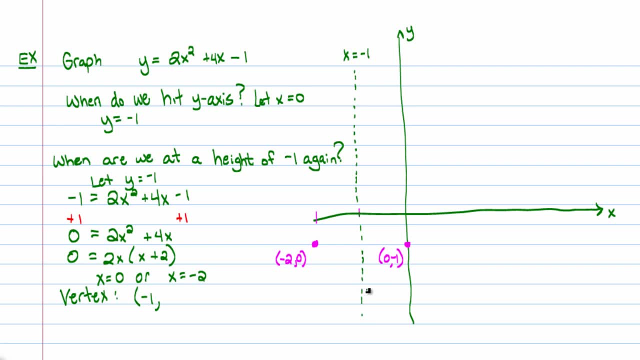 have to do to find the actual height of that vertex is plug negative one into this equation. i'll do it over here. y is equal to two times a negative one being squared plus four times a negative one minus one, that's going to be two times one. 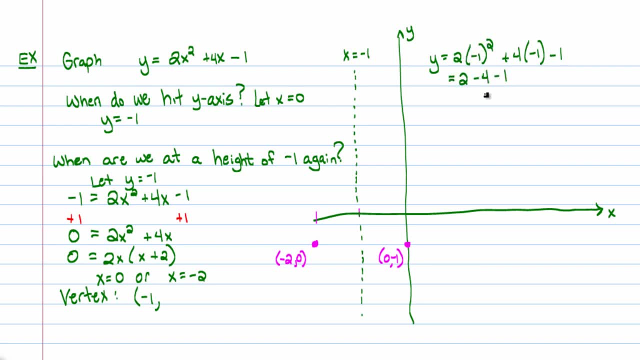 minus four minus one. uh, so that's a negative three, i think right. two minus four is negative. two minus another one is a negative three. so i am- uh, let me do the right color pen here- negative three. so my vertex is at negative one comma, negative three, which all says right here. 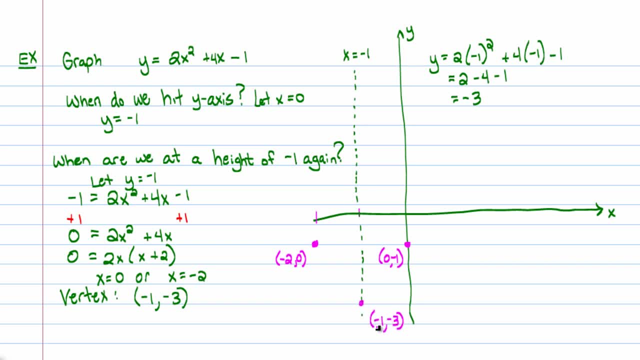 negative one comma. negative three. now i have my three points. i'll connect them up and draw my parabola. okay, now, something that i'm not going to mention in this lecture, but something that might be necessary for a future lecture. uh, just to let you know, because i'm not really concentrating. 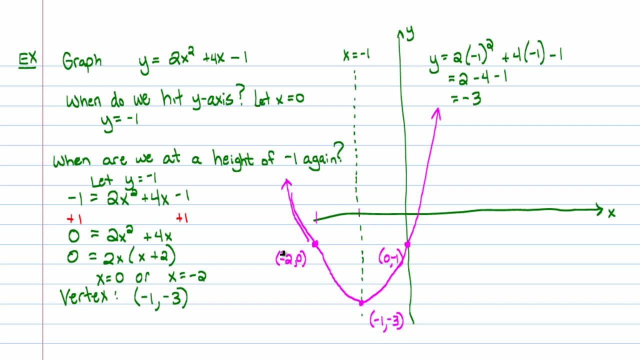 on finding x-intercepts. right now i really just want to know how to graph a quadratic equation. i don't really care about uh x-intercepts. right now i want to know about y-intercepts. the symmetric point halfway in between is a vertex. but later on. 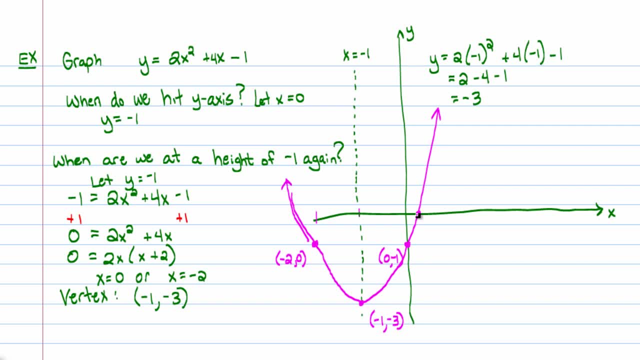 we'll talk about in a future lecture about finding these x-intercepts, but that's not my goal right now. i'm just going over the basics of graphing a quadratic equation. by the way, this is the best way i found to graph a quadratic. there's, i don't think, a single flaw with using 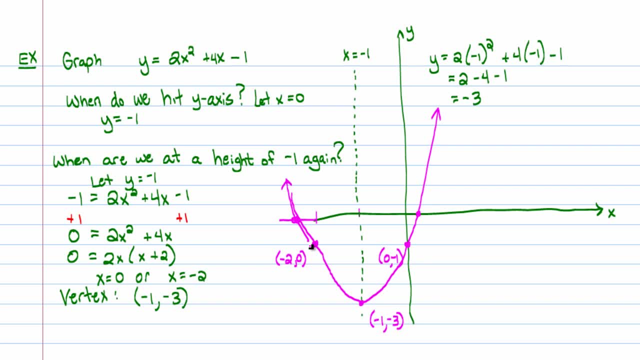 this method because it makes sense, right. every parabola hits a y-axis and every parabola, if you hit, if you reach that height here, you got to reach a height. that height again, because it's a u-shaped curve halfway in between those hits, is going to be. 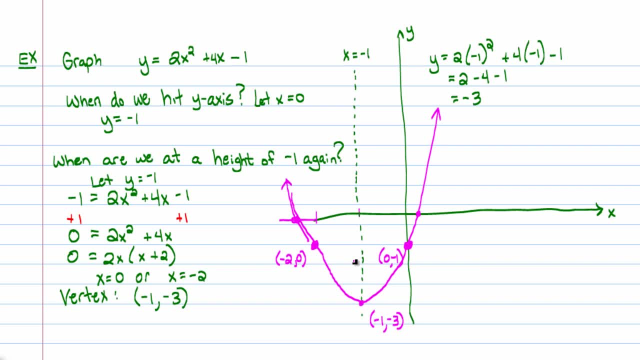 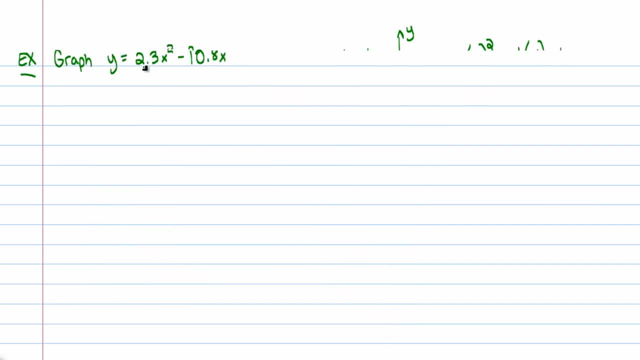 the vertex, that's. i mean, that's as simple as it is as far as thinking. let's go ahead and do just one final example. i just want to show you that you can even use this method to graph a quadratic equation. when you're graphing a quadratic equation with with decimal coefficients- maybe i won't make this- 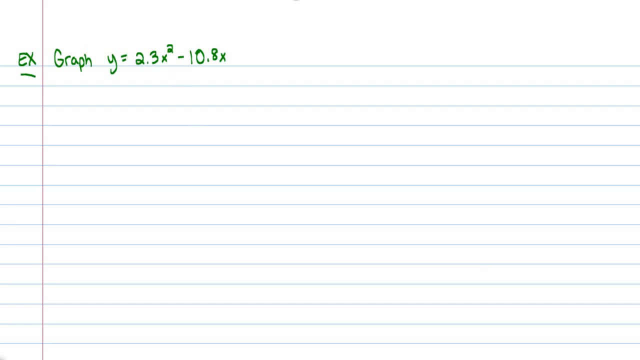 my last one. i'll do one more beyond this. just for those who are using the internet to search for how to graph quadratic equations, they might want to see one that involves an extra plus c here. so do one more of those. i draw my axes in and i'll 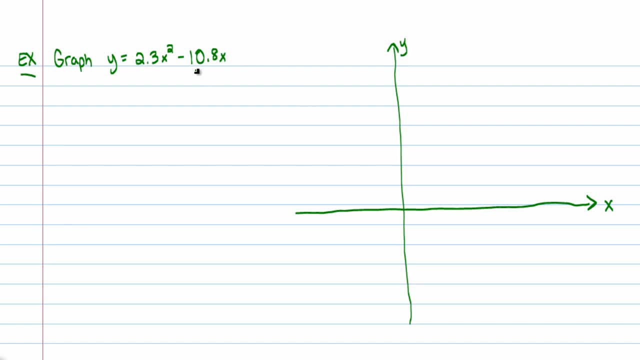 do that, and i'll go ahead and make this one. if you look at this method, you can use it basically just like a regular formula, but i do want to make it a little more simple. what i'm going to do here is to go ahead and mention right now that it's a parabola, right? 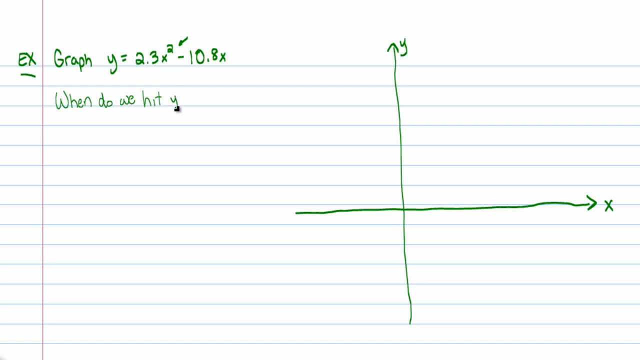 there's the power of two, and all parabolas hit the y-axis. so i'm just going to ask: when do we hit the y-axis? that means what is our y intercept? so let x equal zero. what's nice about this method? there's so many things are great about this method, but another nice thing about this method is i don't really have to. 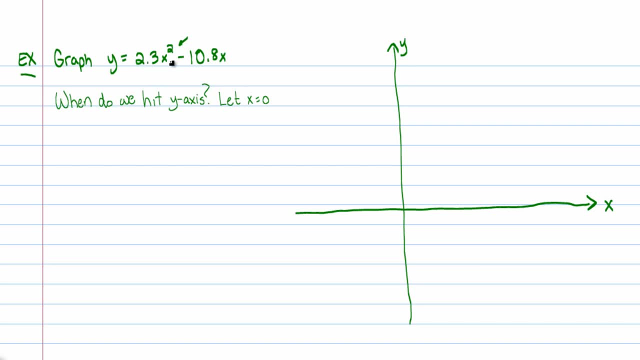 have to deal with decimals. that often here, When I let x equal zero, you see that y turns into zero. so that's a very nice result that our y intercept essentially is zero, zero. so I'll just graph that in there. Now I'm going to ask that question because if we reach a height of zero with this, 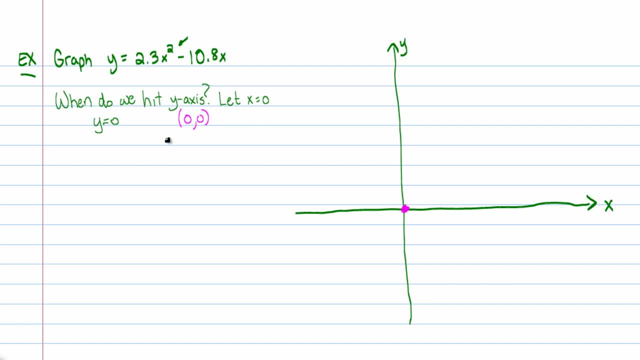 parabola. when are we going to reach that height of zero again? When are we at height equals zero again? I'm just quickly writing it. So if I'm asking you when my y values are zero again, that means let y equal zero. and remember the only reason why I'm letting y equal zero is: 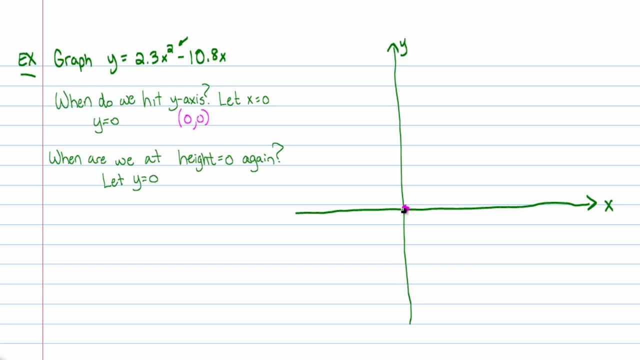 because of the fact that we're going to reach that height of zero again. So if I'm asking you, we found out we hit the y-axis at a height of zero. It's not that you always let y equal zero, it's that you let y equal wherever the value of wherever you hit the y-axis. We just happen to. 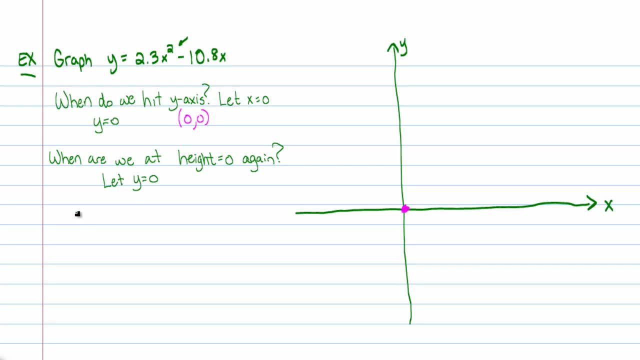 hit it at a height of zero. So when are we at the height again? Well, letting y equal zero, we get. zero is equal to 2.3 x squared minus 10.8 x. In this case, I don't want to factor these decimals, but I 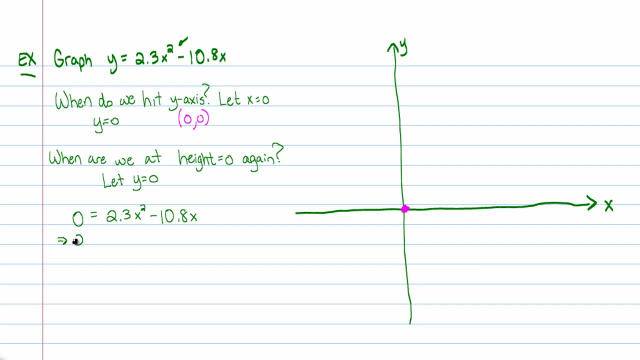 want to factor out the x at least. So I'll factor out an x and I'm left with 2.3 x minus 10.8.. In other words, I'm at that height of zero again, when either x is zero or when, from this, x is equal to 10.8 divided by 2.3.. This is horrible notation. 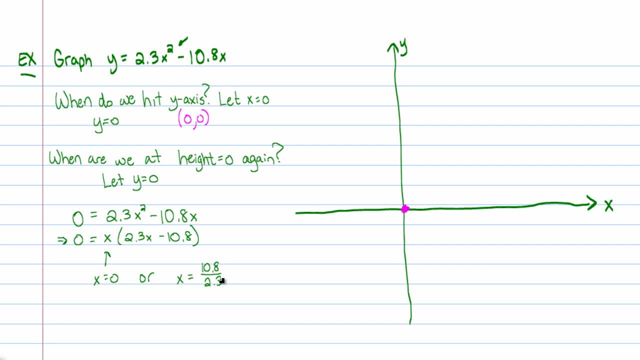 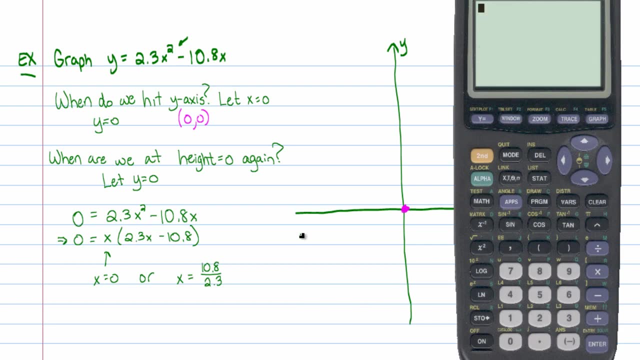 I'm just letting you know. Usually you do not want to have the notation that you want to have, So I'm going to find a notation of decimals inside fractions, because fractions are defined to only have integer numerators and integer denominators. So instead I'll go ahead and use a calculator here, because these are 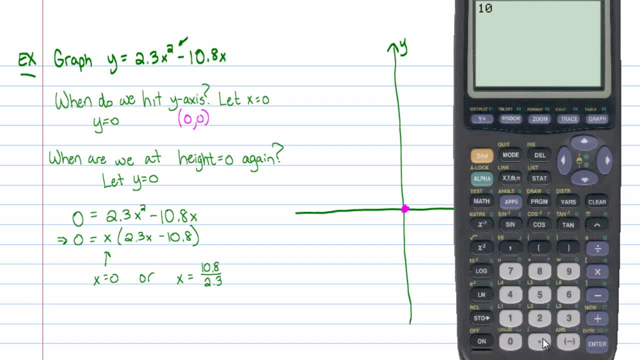 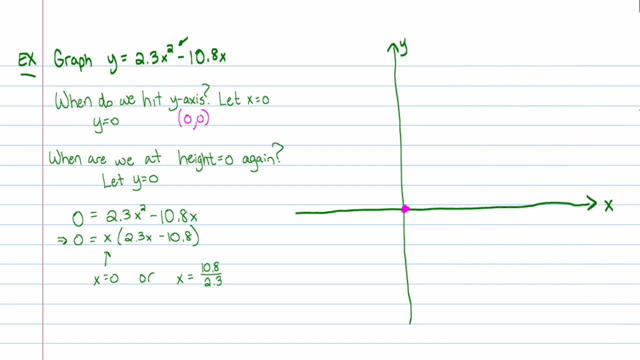 given to me in decimals. I might as well use a calculator to do the division. So I just grab my handy dandy graphing calculator here and I find out this horrible number. Alright, but I'm going to keep that number available. 4.7 roughly, so let me just say it's approximately 4.7. i can still do the math even though i have an. 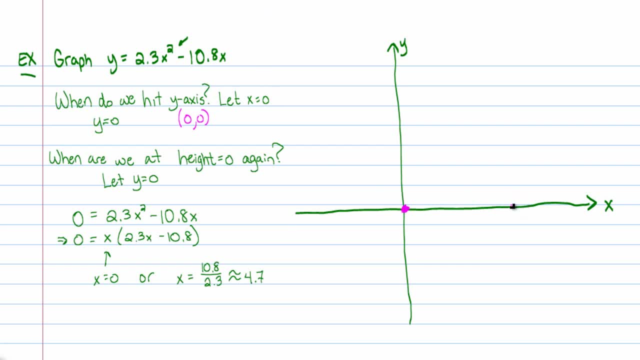 approximate number. now, remember i'm asking: when am i at a height of zero? so that occurs at x equals roughly 4.7. so i'll just put that in here. 4.7 comma zero, halfway between these two points, is going to be my axis of symmetry. i'll graph that in in purple here, halfway in between. 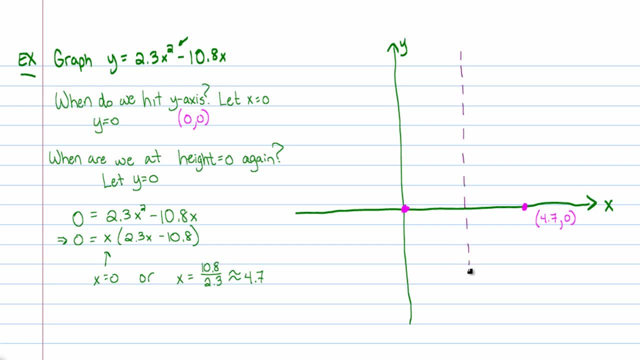 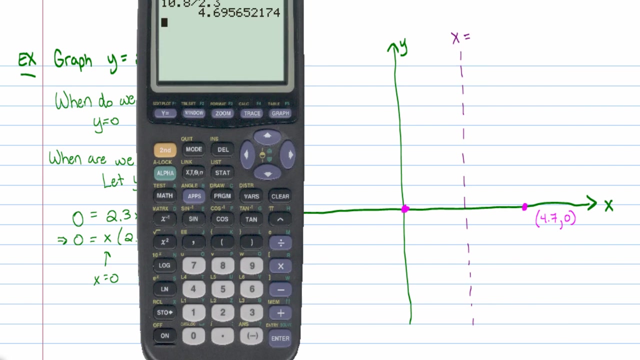 that looks almost halfway. i kind of went a little bit too far to the left there, but whatever, and remember it's a vertical line, so it has an equation: x equals and it's halfway in between 4.7 and zero. i'll go ahead and drag the calculator over and just say: divide that last number by two. 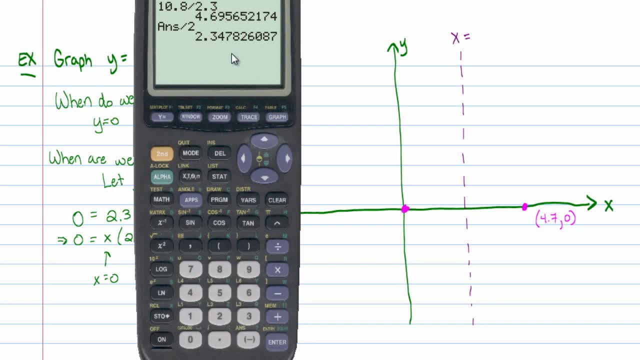 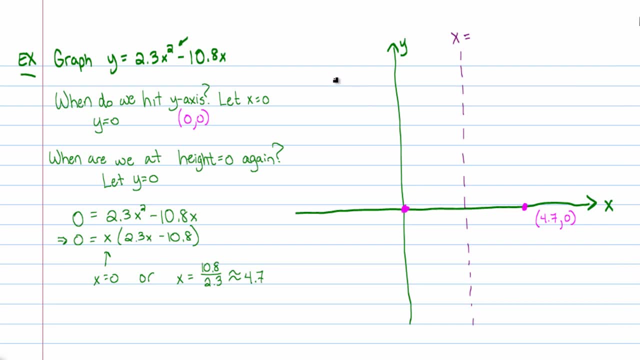 because that's really the halfway point and it looks to be about 2.3 five. so i'll write that in there. 2.35, that's very roughly. we've approximated that value, but still it's okay, because i now know my vertex is approximately. i'll write that in. vertex is approximately. 2.35 is the x value. and now i just 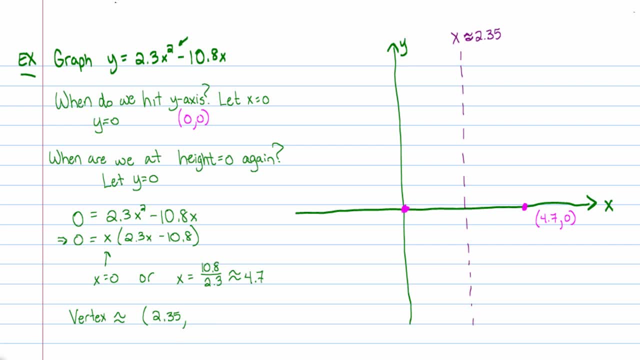 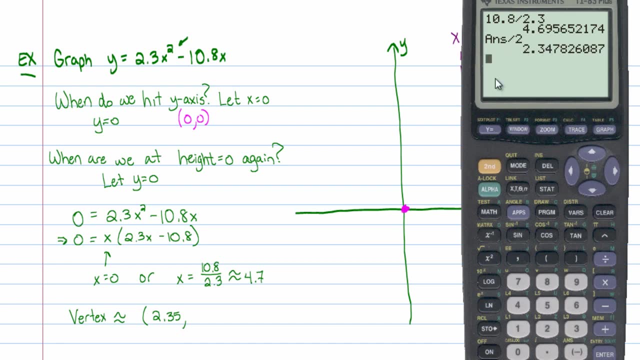 need to find the y value, and i'm going to do that, and i'm going to do that, and i'm going to do that value. and because i have a calculator right here and i have this number already ready to go, i'm going to go ahead and teach you. if you have a graphing calculator, teach you how to store that. 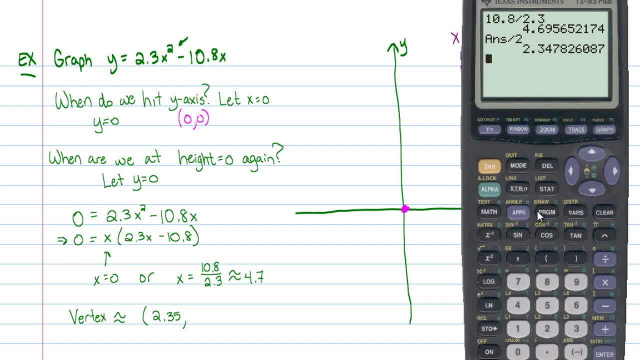 number. if you don't have a graphing calculator and you can't store it, well, you're just going to have to basically say what's 2.3 times 2.35 squared minus 10.8 times 2.35. for those who do, 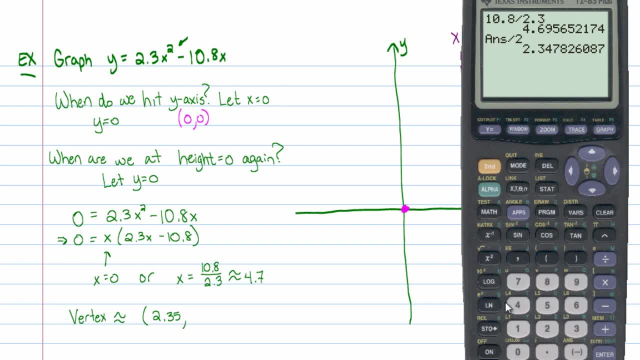 have a graphing calculator. i'd like to teach you a trick. if you get an answer and you want to keep it, you can hit this sto button. that means: store that please, and you have to select a letter. you're going to store it as well. you have every letter of the. 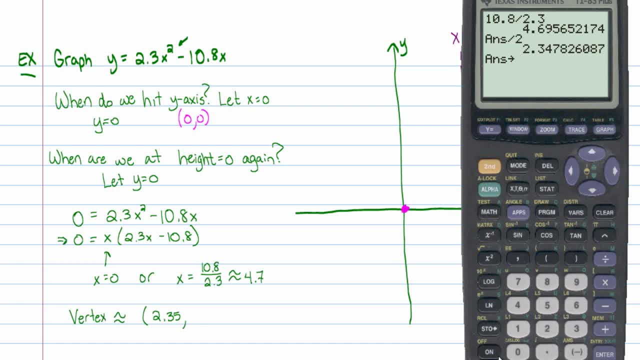 alphabet available. i would. i don't know why, but i would just probably avoid using x. i usually just store it as a, so to access the letters, you use this alpha button, click alpha, and you see you get this blinky little a there. and now, anytime i press a key on this keyboard, it'll actually 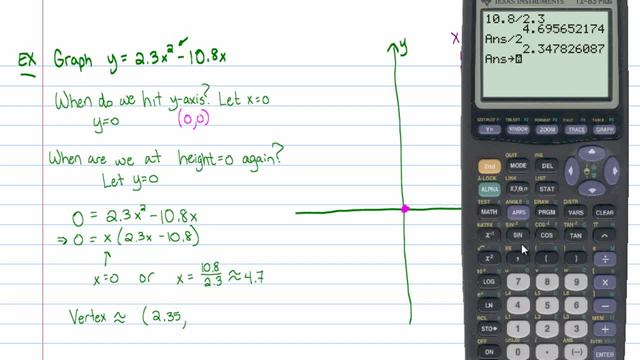 replace the letter that's in the alphabet. so i'm going to go ahead and do that and i'm going to use this, uh, this blinking cursor with the letter associated with that key. so if i want a, i'll just hit the button that has the little green a above it. so i've stored that answer as a. now what i'm? 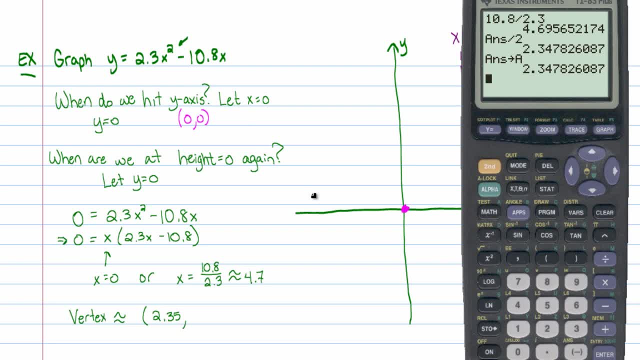 going to do is find out what 2.3 times a squared is. 2.3 times technically. you don't even need the times a squared, well to remember. to get the a, it's alpha. and then a squared minus 10.8 times, again alpha. a notice: the same format right: 2.3 x squared minus 10.8 x 2.3 a squared. 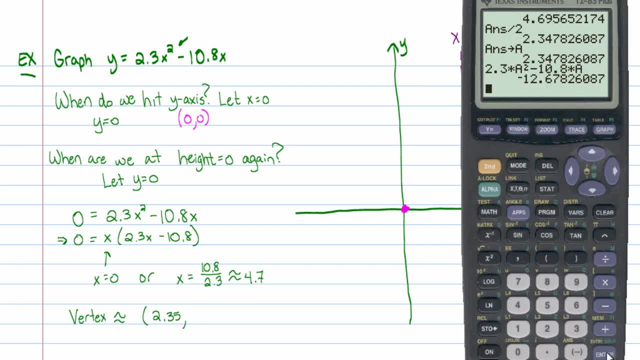 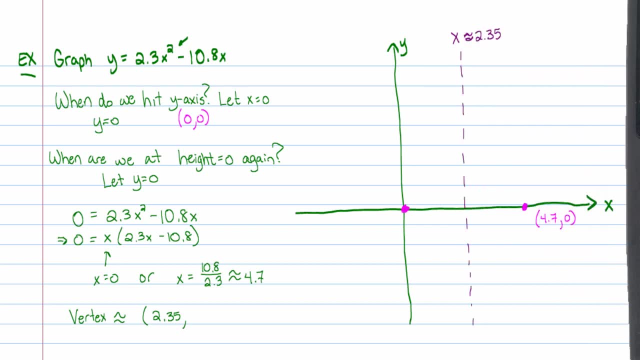 minus 10.8 a and you get a negative 12 point. and i'm just going to round the nearest, uh tenth here. let's go negative 12.7. that's pretty far down there, uh. so i'm just going to pretend as though it's it's right about here, and that's uh four point. eight times again alpha a and then 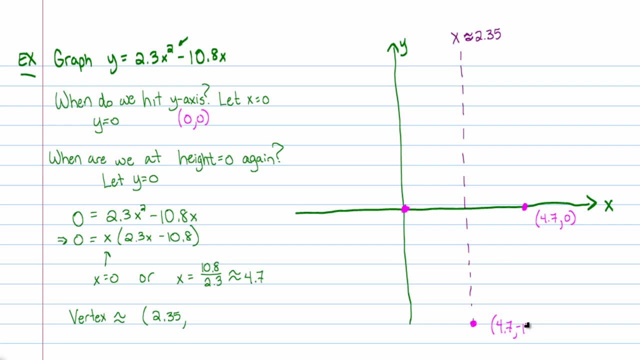 negative 12.7, comma negative 12.7, and i should probably write that in also here: negative 12.7. now, once i've done that, i can actually go ahead and graph the rest of my parabola. wow, that's the best curve i've done all day. 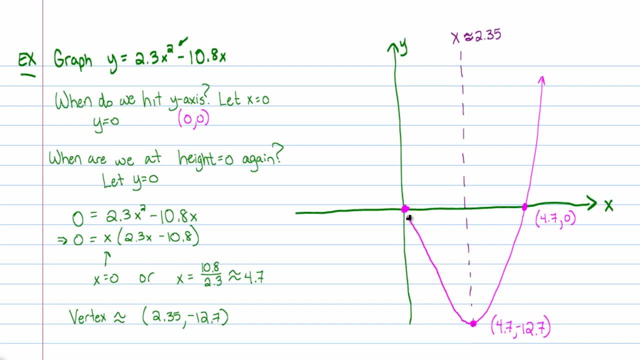 and i will mess it up by doing that. okay, it's supposed to be symmetric, but it's a little bowed on that side. okay, and there we have it. we have our parabola graphed. even though it's some messy looking numbers, it gets graphed. now to show you the power of this. 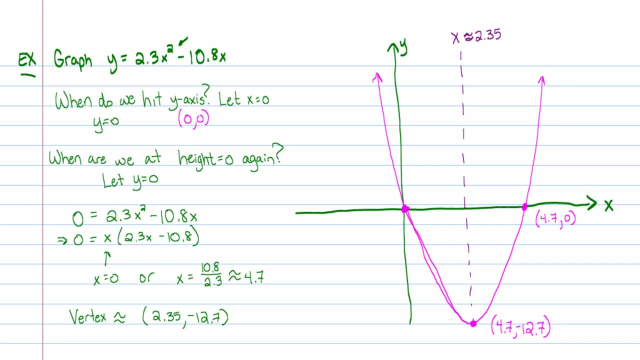 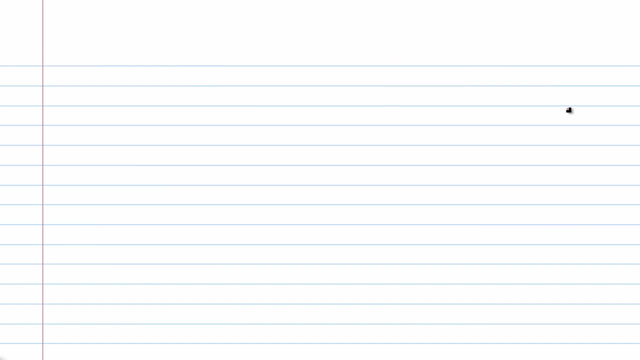 method. i'm going to do one last example, and this example i'm going to do at near to full speed and it's going to make up a problem, and i'll choose ugly numbers too. i'm going to basically because i can go any speed i want. you can pause the video, so i'm going to make up just some ugly. 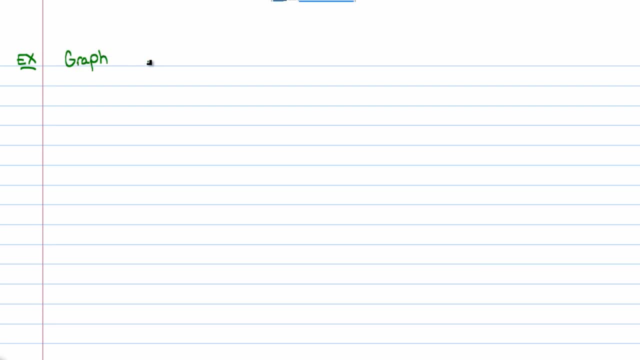 numbers here, graph y, and i'm going to do one last example. so i'm going to do one last example, so i'm going to do a negative. let's do one third x squared minus two-fifths x. uh plus um, let's do a plus. i don't really care. 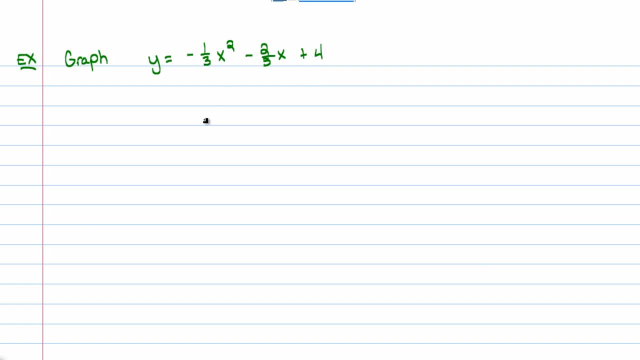 plus four. let's do a plus four, all right. so i'm about to go full speed. let me just get my pens working. i know it's got a y intercept, so y intercept, let x equal zero. y will be a positive four. i'm just going to quickly graph my axes by. maybe i'll use a larger chisel on this one. 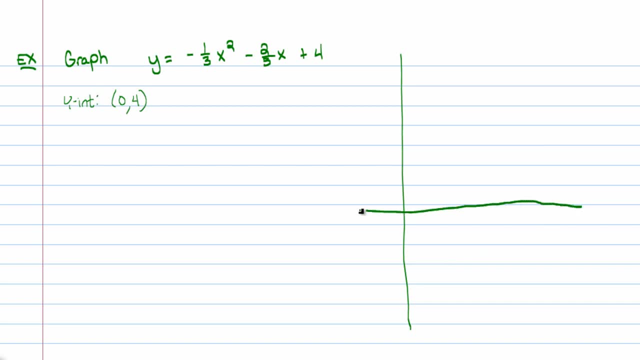 here's the x-axis, here's the y-axis label. all that stuff go back to my regular old chisel here and i said it's at a height of four, right? so one, two, three and four, so it's zero comma four. there's my y intercept. now i'm just asking: when am i at that height again? 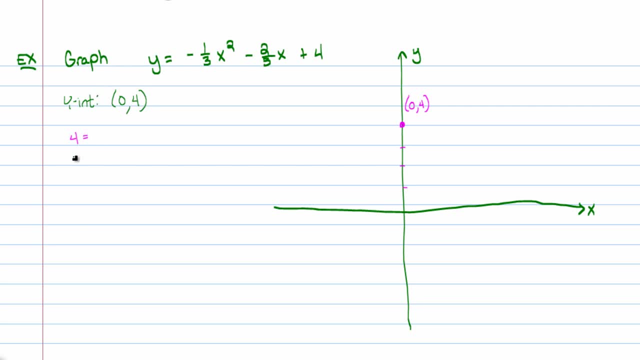 well, that occurs wrong color pen. that occurs when y is equal to four. i just want to know when is y four again? technically it would be much faster than this. even i'm going to subtract four from both sides to start getting everything on the right hand side and lo and behold, i get zero is equal to a negative one-third x squared minus two-fifths. 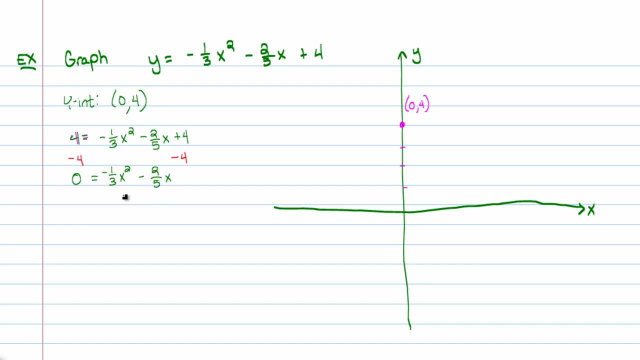 x. notice there's no constant left. great, let me factor this: pull out an x, that's all i really care to pull out. and it turns out that i'm on. i'm at a height of four again when x is zero or when this junk in here is zero. that's going to take a little bit of solving for me. 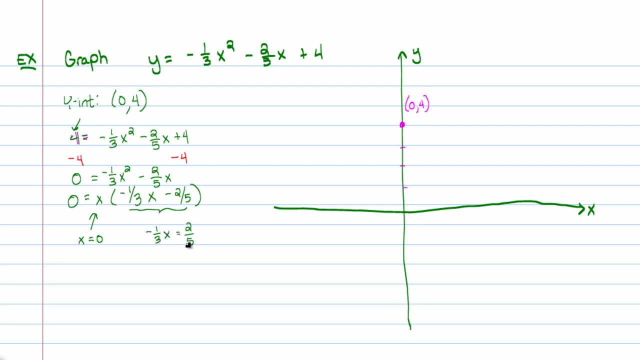 in other words, when one negative one-third x is zero, and i'm at a height of four again- when x is equal to positive two-fifths, multiply both sides by negative three and you get x is equal to a negative six-fifths. okay, that tells me that. 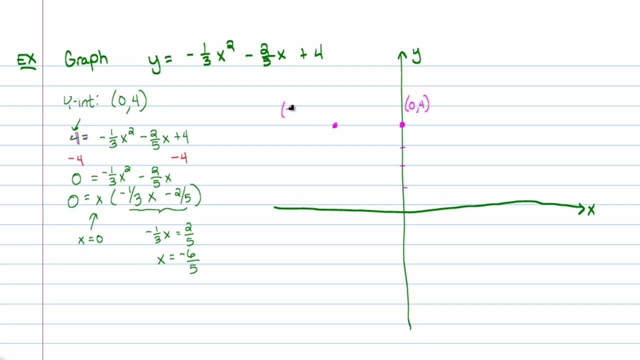 this point right here occurs at: x equals negative six-fifths, comma four, right the height of four. so it tells me i'm at a height of four at when x is zero and when x is negative six-fifths. halfway in between is the axis of symmetry. just draw that in here. 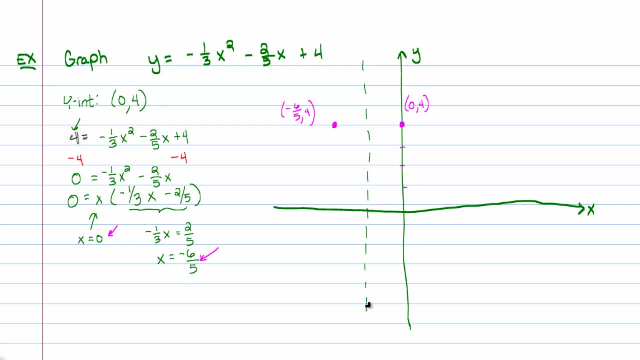 great well, let's see, halfway in between zero and negative six-fifths is actually negative six-tenths. i just multiplied the denominator by two. that's all you really have to do. that's what half of a number is is multiplying the denominator by two. but i'd like to reduce this fraction. 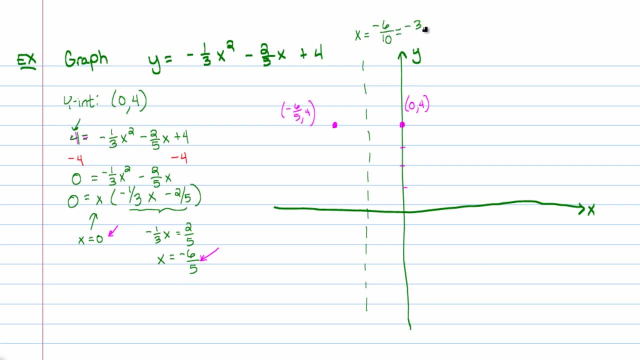 so they're both divisible by two. there's negative three-fifths. all right, know, the axis of symmetry is in negative three-fifths. the hardest part really is this last part. It's finding what the y value for the vertex is. So I'm going to plug in negative three-fifths. 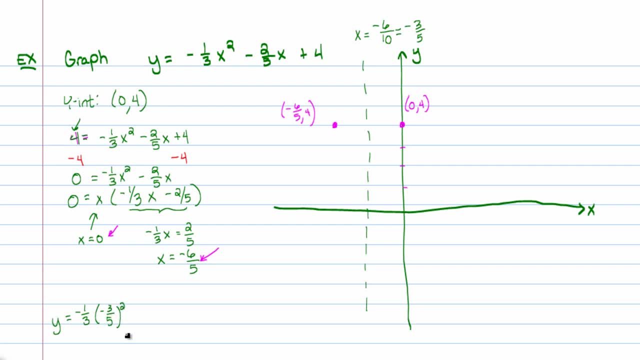 into my equation. This is really the lengthiest part, but you'd have to do this no matter what method you use for graphing. So let's see, we have negative one-third times nine-twenty-fifths. Let's see plus, six-twenty-fifths plus, and since everything looks like it's going to, 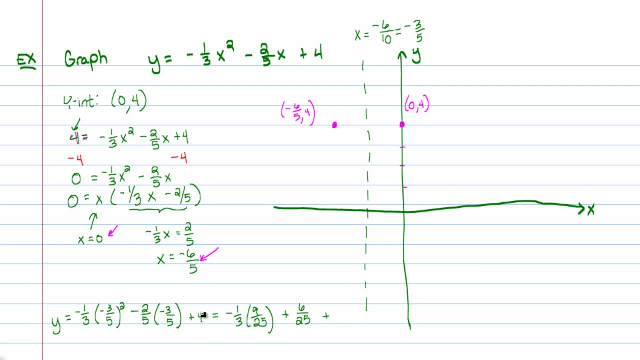 have twenty-fives in denominators. I'm going to change this to be one-hundred-twenty-fifths, Which equals. let's see, three goes into nine, three times, so it's a negative three-twenty-fifths. 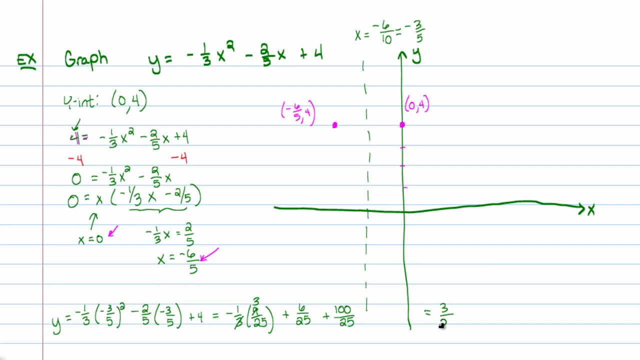 plus nine-twenty-fifths, Plus six-twenty-fifths, that's going to be three-twenty-fifths Plus one-hundred-twenty-fifths, which is going to be one-hundred-three-twenty-fifths. 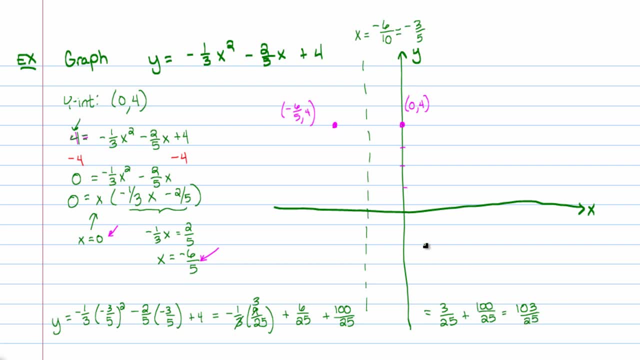 That does not reduce. So one-hundred-three-twenty-fifths, that's a little bit over four actually, So I'm just going to go ahead and plot that right about here. That's just slightly over four, and I'm going to label it first of all so that occurs at. 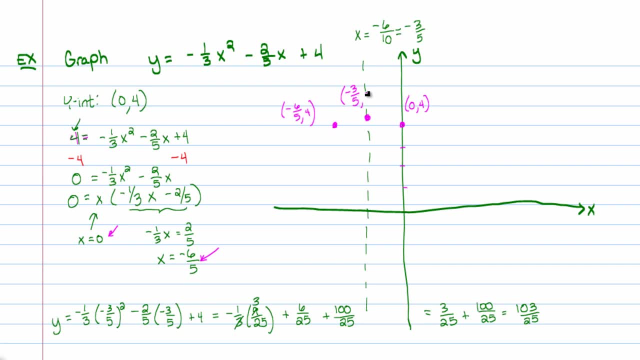 x equals a negative three-fifths. y equals one-oh Three over twenty-five. And now I'll connect these with a nice smooth curve. I'm having a hard time doing that. Make sure if it starts wide, you keep it wide. 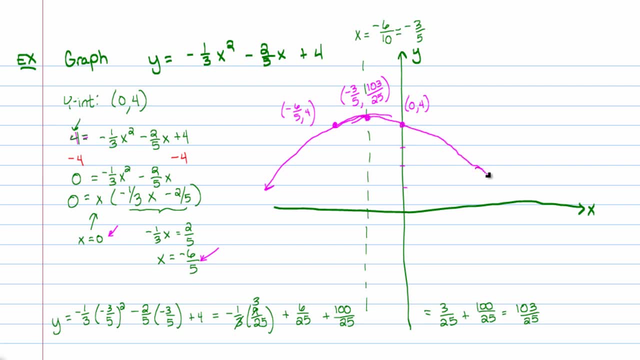 Don't make it just all of a sudden flop down. It should make sense that it's opening down, though, because it has a negative coefficient on the x squared, that means it opens down. I can't resist. I just want to do one more. 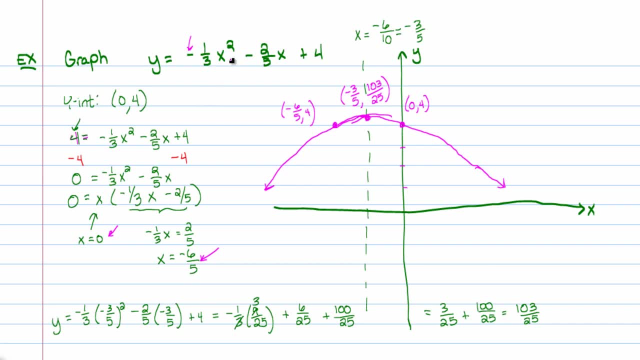 Full full speed, So I will do just one more at full full speed. You can always just stop this video right, So it doesn't really matter, But I just can't resist. I really love graphing using this method. 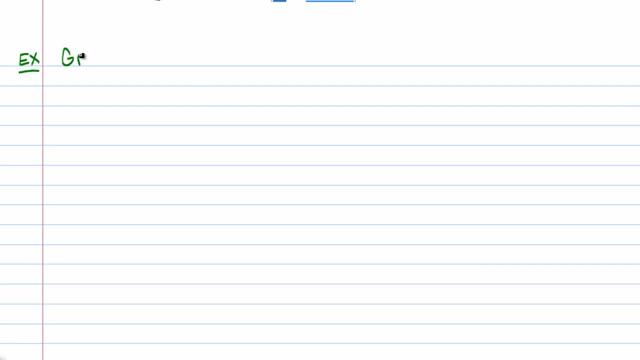 Ridiculous, isn't it? So graph? and this time I'm not going to make it so ugly, I'm just going to show you the power of it. if you go quickly, Three x minus. I'm just going to make my life easy.